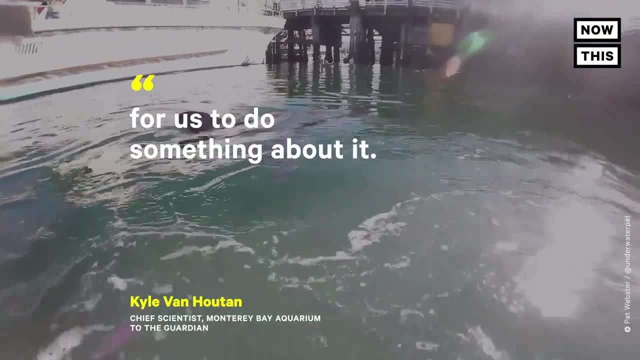 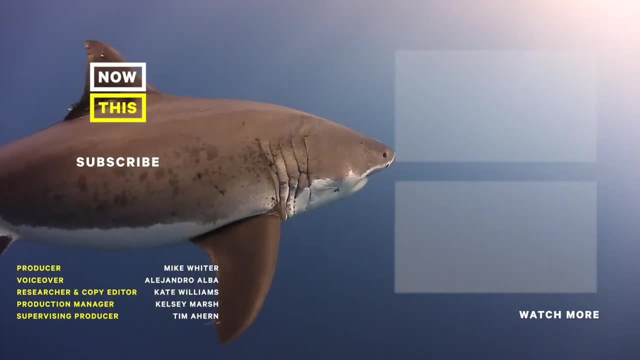 sharks are telling us that the ocean is changing and it's now time for us to do something about it. Thanks for watching. 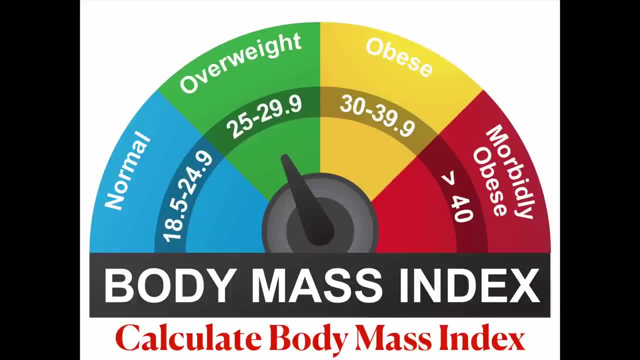 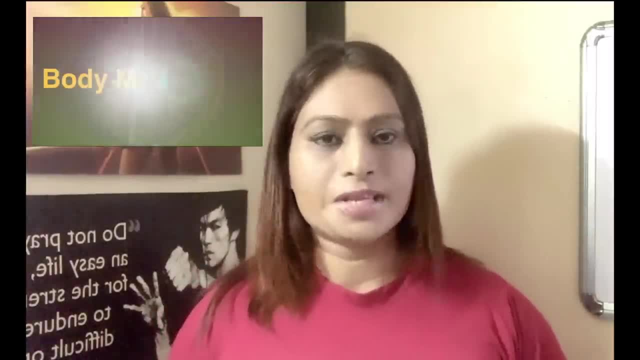 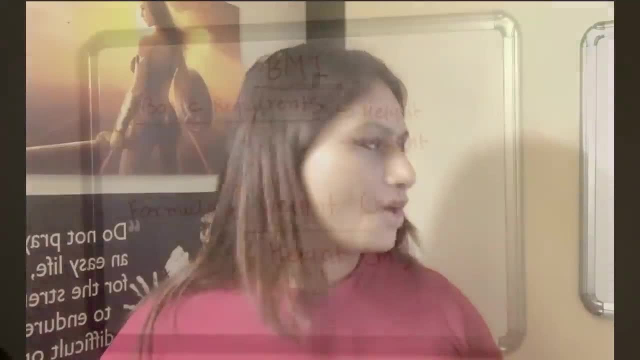 Good morning everyone. Today I am going to talk on the BMI and calculation of BMI. What is BMI? The BMI is a body mass index and it is one of the major to find out the fat percentage in a human body. So let's see how it is. First of all, we need to understand 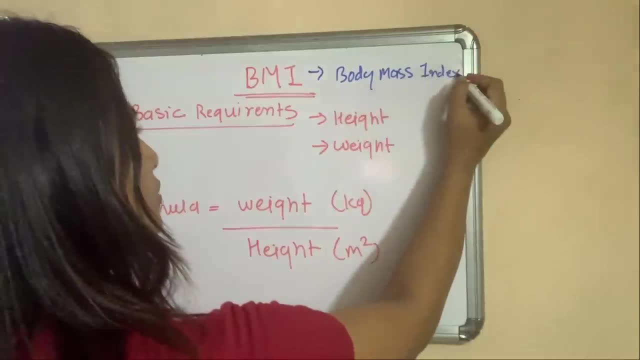 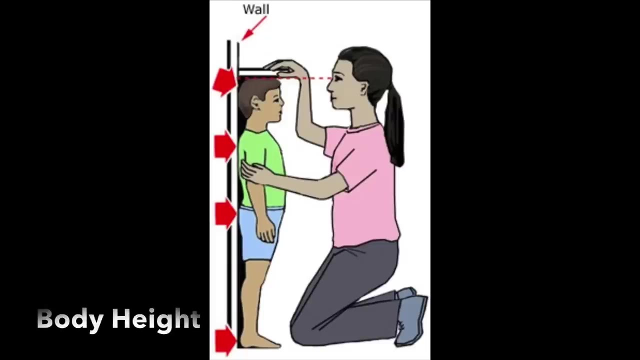 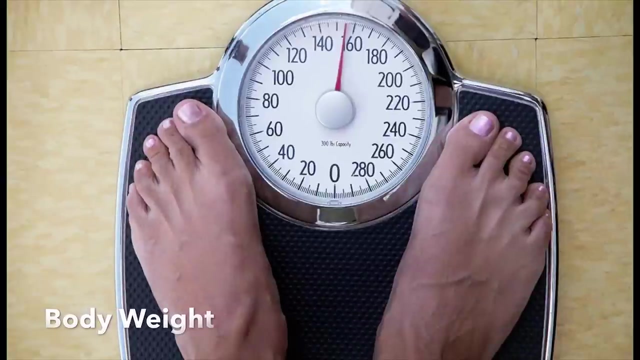 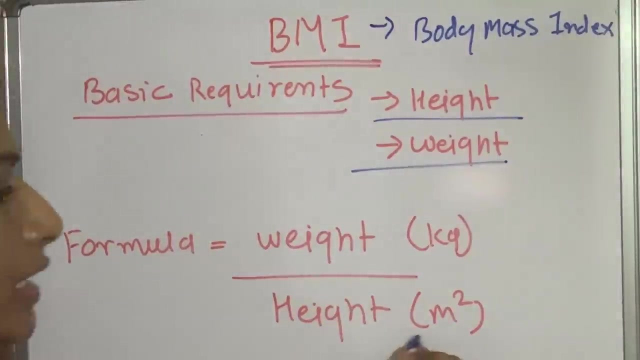 what is requirement for the BMI. So we need two majors for the BMI. One is a height and another is a weight. This is the formula of BMI: The weight divided by the height in the meter square. So generally we calculate our height in the centimeters, but then we 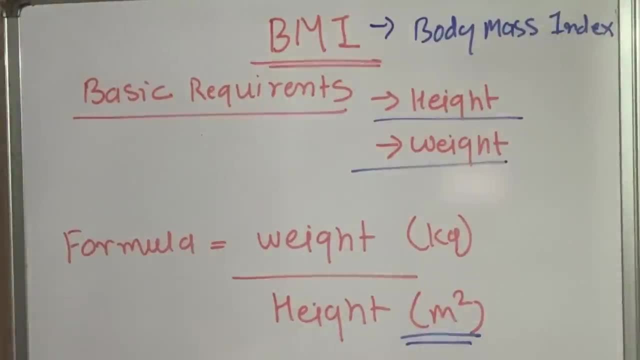 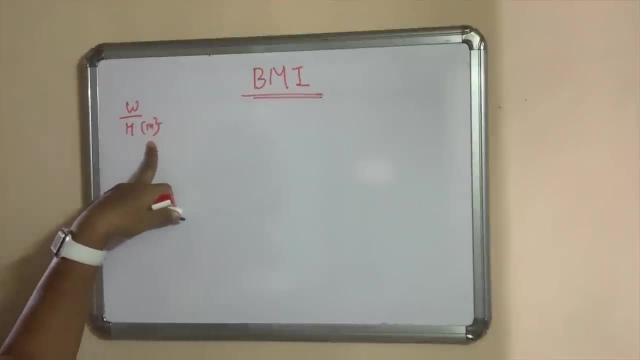 have to convert the height into the meters. How it is, we will see that To understand the meter square, because generally we measure our height in the feet or the centimeters. So if I have a height in the centimeters, So how to convert that centimeter into the? 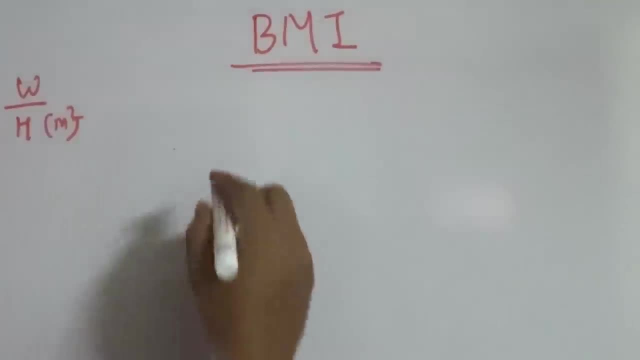 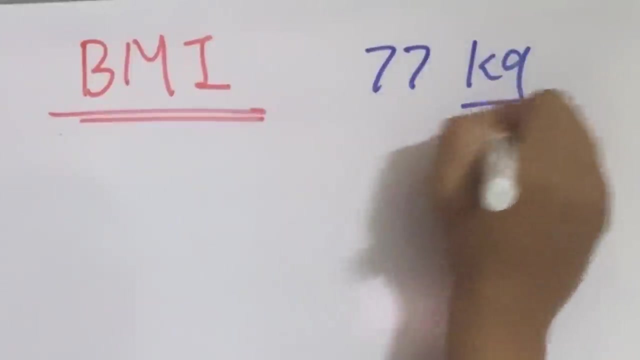 meters. So it is very easy to calculate that 100 centimeters equal to 1 meter, Right, Okay, let's take an example. Somebody has 77 kg weight. Seventy seven kg is someone's weight- and suppose its height is 165 centimeters. So if I have a height of 165 centimeters, So 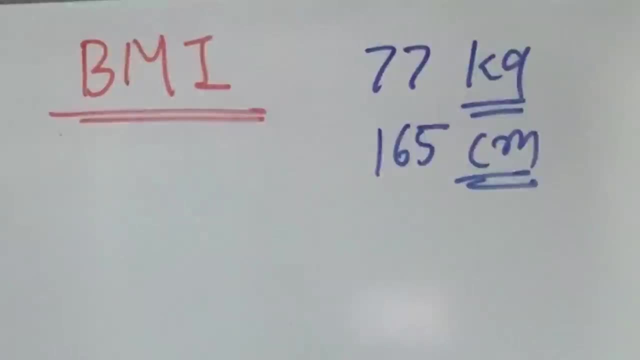 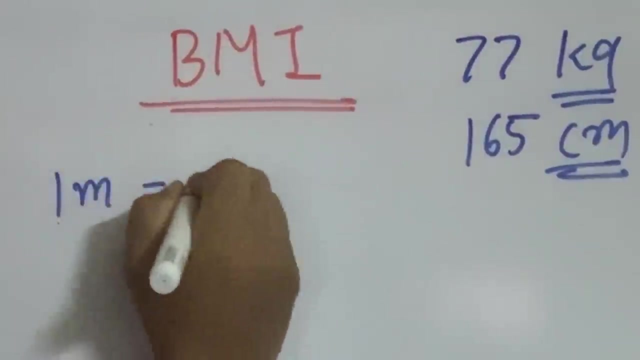 it is a centimeter height. Now we have to convert the centimeter into the units of meters. It has a very simple formula: 1 meter equal to 100 centimeters, Right? So 165.. What will happen? These two digits will come to the back, and then 165, which will be centimeter.